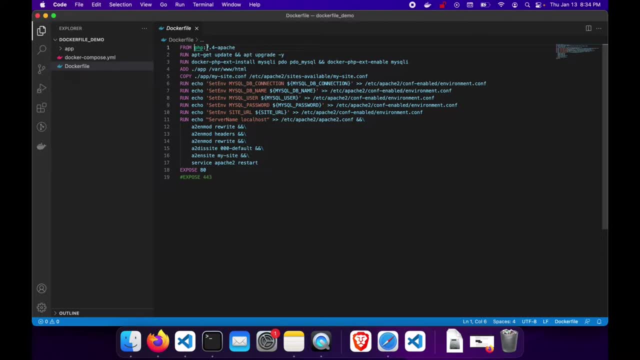 From Docker Hub, I believe it is, And it's the 7.4 Apache version. Basically, the way it works is that you can dockerize any PHP application, But this one's going to be for a web server. So what you want to do is this: actually provisions a little Linux instance and then it runs through everything that you want it to do, So you can specify anything you want here. I have some examples for connecting to a database connection. 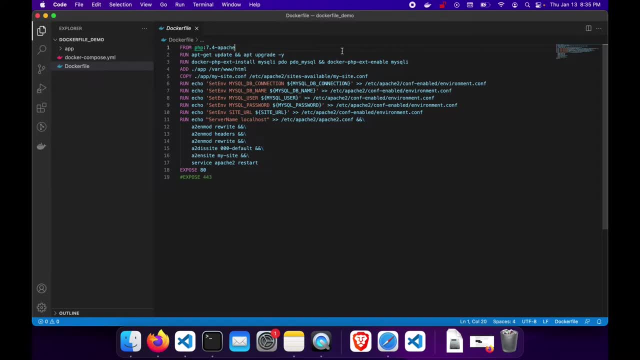 Including the modules that you're going to need for your application to work once it's running in Docker. So good rule of thumb is: anytime you're going to be dockerizing anything, you want to run apt, get update and then also upgrade. because you're going to be pulling down a vanilla Linux instance And you want to just upgrade everything and update it so that you can pull anything you need. So here we have run Docker. 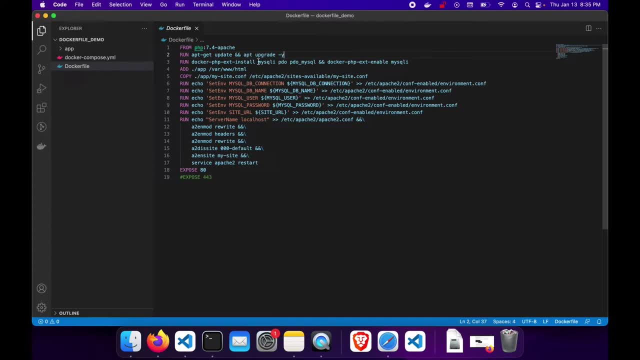 PHP extension install, And then we have a list of modules that we want to add. You can see here that it's my SQL I. you can also do the PDO extension, And so if you know what extensions you need, go ahead and throw those in there as well. And what we're doing here is we're going to add the our, our app directory, all the information in there, into the Apache web server directory. 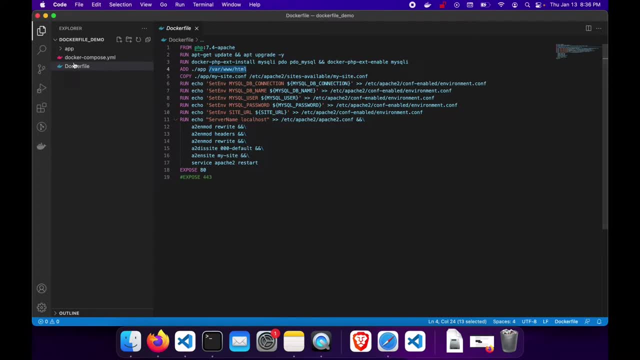 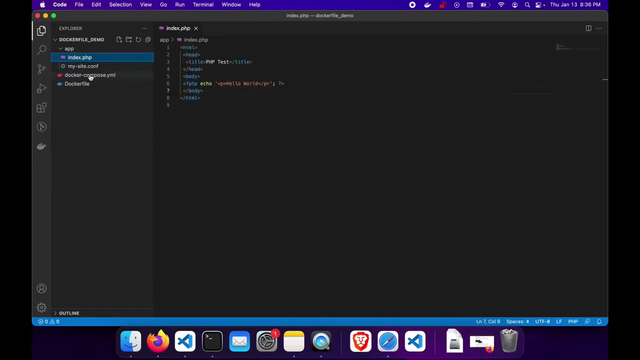 So that's VAR WWW HTML. So it's going to be going into this folder right here and then grabbing everything and copying it into your Docker image. So then we're also going to copy over that configuration file. So in here you can have your, you know, redirect rules and everything that you need in there, and it'll actually copy it over to the application So or to the site, And right here you specify the name of your site. We're not going to use the default site. Generally good rule of thumb is to use the default site. 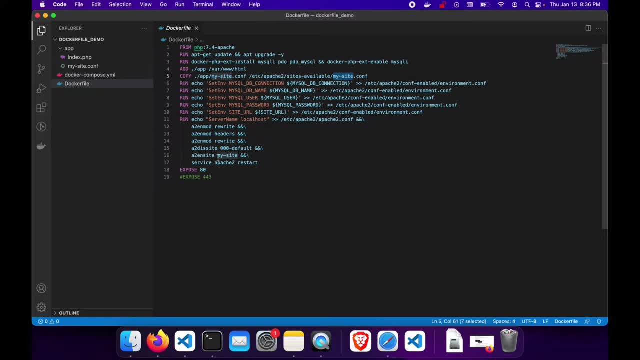 We're not going to use the default site. Generally, good rule of thumb is just to not use that. Down here it's also defined, So be sure to update this as well. Also, so you're able to actually set environment variables when you provision these Docker instances, And this is helpful especially when you're trying to have, you know, multi container deployments with separate connections. you're making API calls to different, you know domain hosts and all of that kind of stuff. So for here, this was the use case that I had, So I just wanted to. 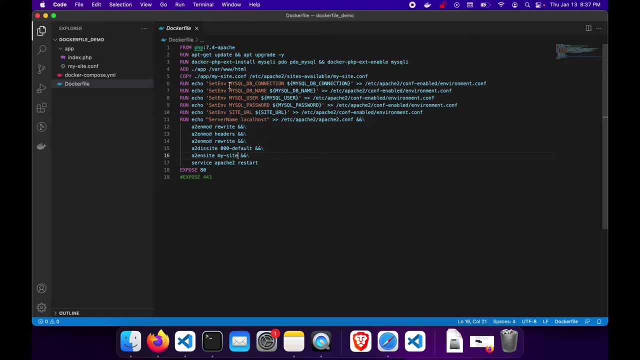 throw this in there. We have these Docker containers that are going to be connecting to multiple SQL database connections. So what I'm doing is I'm actually setting an environment variable, or I'm actually like setting up to you or to add an environment variable to what I need. So, basically, all we're doing here is we're echoing this command And then this will be passed in when we create our Docker composed file, which I'm going to show you in a little bit. And then these two slashes mean just whoops, these. 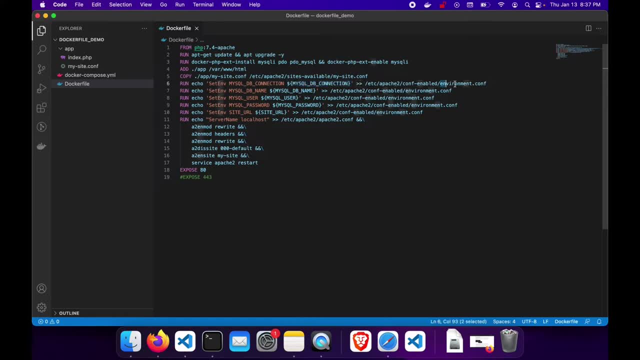 two slashes mean: just append the environment configuration files So you can go ahead and add whatever you want here. just be sure to name it what you need And then also give it a good name, usually the same name, so that you can reference it in your Docker composed file. Okay so, and then also down here we have some commands. Basically, what we're doing is we're provisioning from the default site And we're adding this site name that we're going to be using. 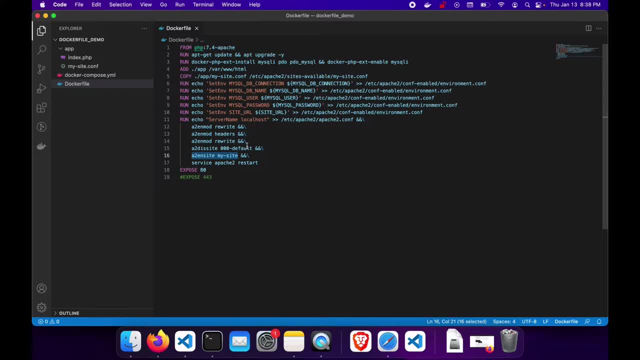 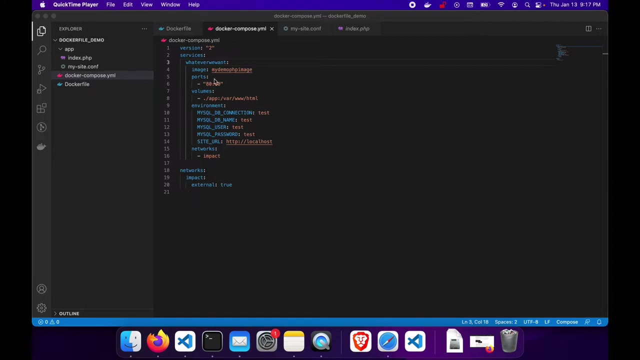 and that's why we have to update the configuration file site name here. And then we're just going to restart the Apache service And I'm exposing on port 80.. Because this application is going to be running behind an application load balancer And there's no need for me to expose on 443.. I just have this on there just to show that it's possible. Your Docker composed file. we're going to be using this to run the Docker container locally. So here we have just a list of 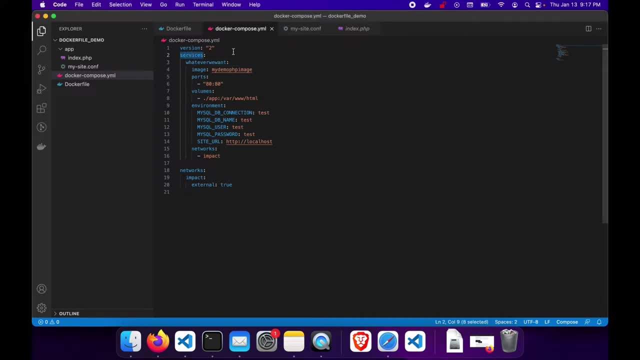 servers. This is what YAML looks like. this is how you can basically statically run containers. So rather than having to, you know, use Docker run and specifying your ports and all that, you can just have a file that does it and then just run off of that file. So here we have just a service name. this is used to reference across your file. you can name this absolutely whatever you want. It doesn't matter what you name that. 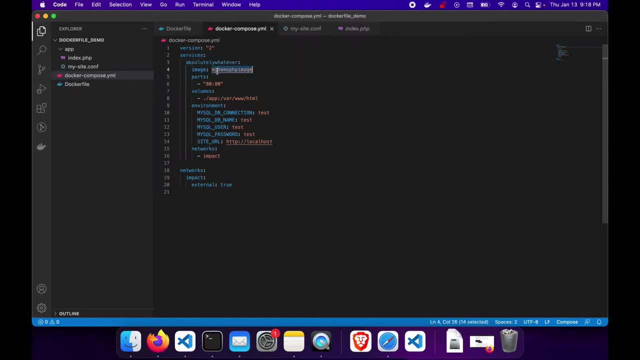 Here we have our image and it's going to be named my demo PHP image. you can name this also whatever you want. just make sure that when you're building your image you're building it that same name, because this is going to be pulling that image that you build later. So for your ports here on the left side, you can specify whatever port you want to specify. you can do port 8000,, you can do 3333,, it doesn't matter. 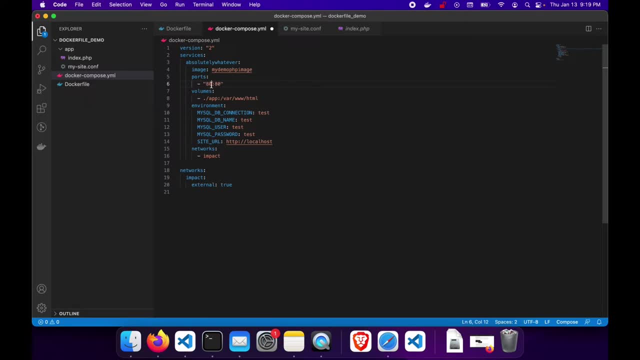 I just use port 80, because when you type in localhost, it automatically goes on port 80. This side is where it actually hits the Apache web server service. So just keep in mind, on this side it's going to be port 80, almost always. So you have your list of volumes here. This is helpful if you're not trying to build your image every single time that you make an adjustment or a change. 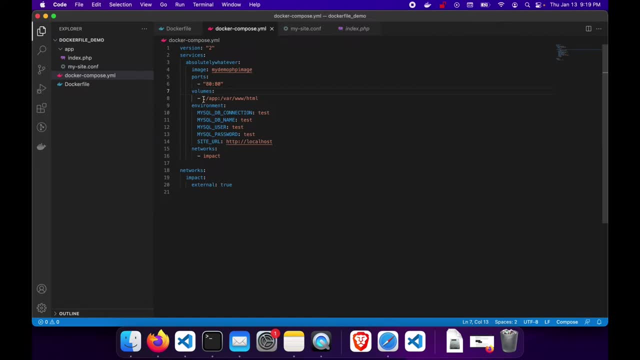 So you have your list of volumes here. This is helpful if you're not trying to build your image every single time that you make an adjustment or a change. So what this is doing here is this is saying: go into my local directory, go into the app folder and then specify this as our web server. So similar to how you have in the Docker file where you're building the image. you're doing the same exact thing, But here it's going to run locally, no matter what. So we're going to go ahead and remove or comment this out for now, because we're going to be actually running off of our 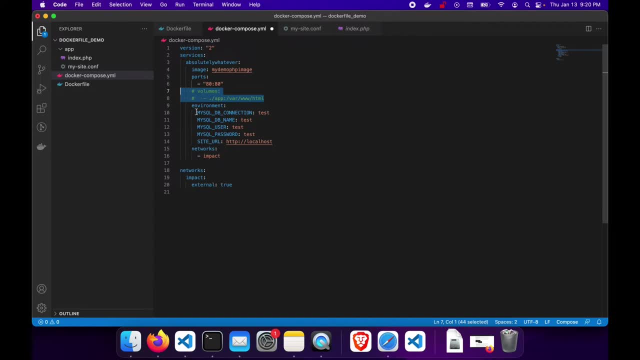 Docker image that we create. You have your environment variables here And all you have here is the same environment variables that you have specified here. So just make sure you use the same casing and spell it correctly, and all that, And then you can just reference whatever you want as the values. So an example would be: you know, an RDS instance, the host name, and then here would be the name of your database and then the username. 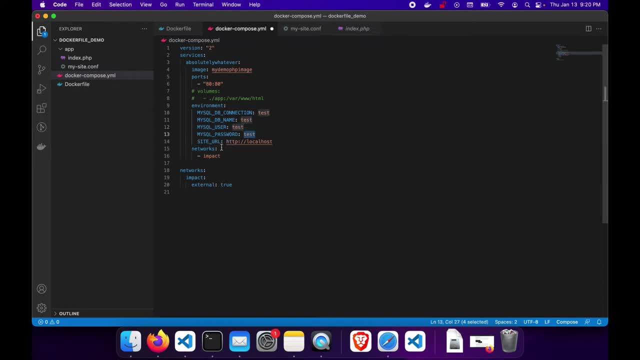 And then the password to the database. You can also have stuff like site URL, which is something. I named this, all the stuff on this left side. These are all names that you can give. It's just you have to make sure that the references to them are the same value. I was using this specifically because I had, for one instance, a dynamic subdomain routing situation And I needed this to be dynamic. So I'm just labeling this local. 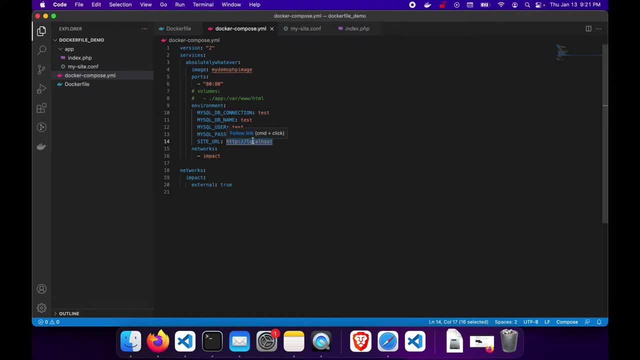 host. it's not getting used in this application. I just wanted to show you that it was possible to do that. And then you can also have network specified, And this is really helpful if you're running a local SQL database instance And you want to connect to it within the same little local Docker network. What you want to do is just go ahead and create a local Docker network and then just specify it as an external network. That way when your Docker compose runs, it knows that that network is 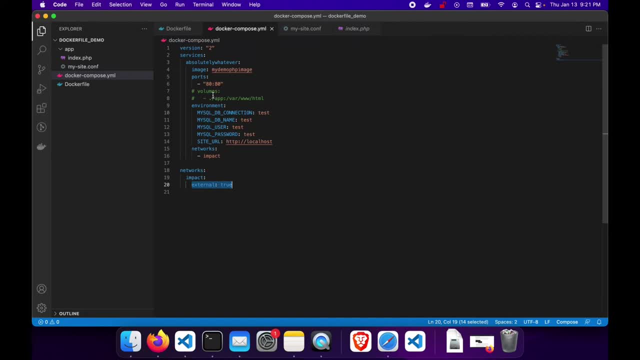 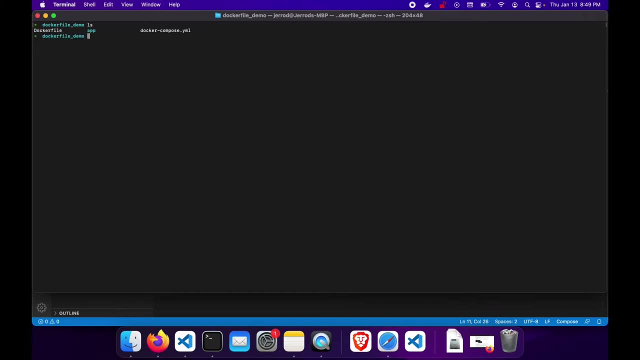 doesn't already exist and it goes ahead and it or the network already exists and then it connects to it. So back over to the terminal. we're in the same directory that we were in in VS code And we're just going to start by building our Docker image. it's really simple. you just have to run Docker build dash T And then we're going to use the image name that I had given it in the Docker compose file And we're just going to run that in this directory, which is the dot. 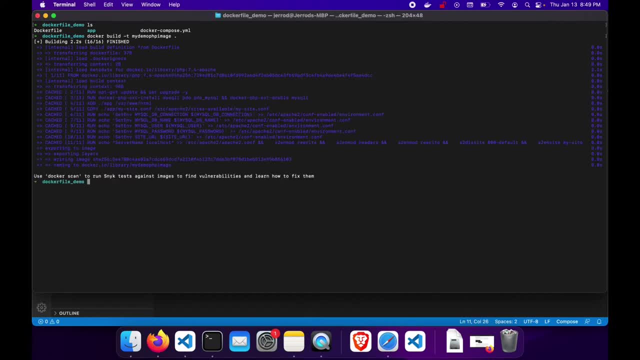 website And then I'm going to just say my image and then print. I'm just going to copy that. Alors, okay, so now you can run your Docker image And basically we have a Docker compose file that we had created. I'm going to just go ahead and show that the image was created running Docker image LS and then I'm just going to Market shepherd. 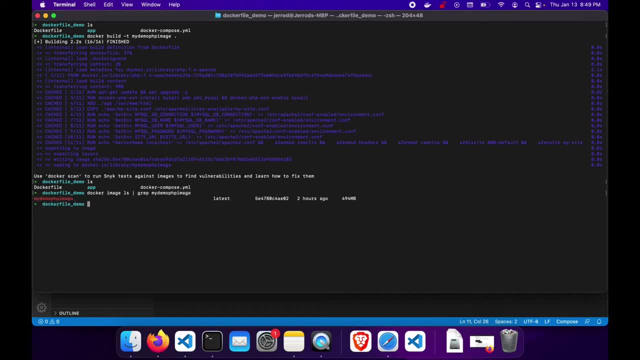 grep for that image name, because I have a lot of different images. Okay, there we go. So you can see my demo PHP image has been created, And then you can see my domain. This is what I want this to look like. this image as a demo PHP image has been created, And then all the things that we need to do is to placed. that Isn't just when I'd want to create the document, Seshan. 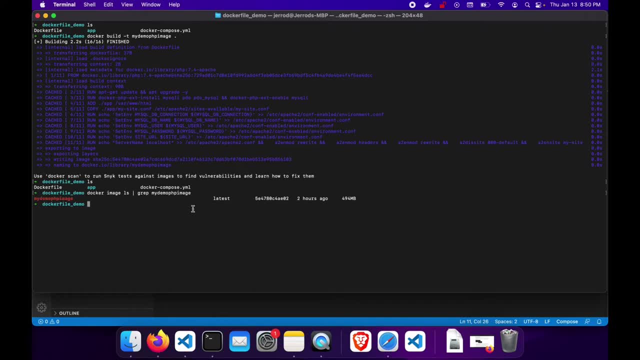 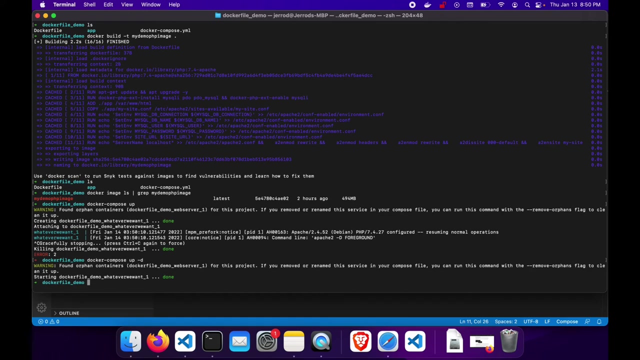 image has been created, so we're going to start by running the docker image using docker compose up. so now it's running. if you want to be able to actually go into the server, you can either open up another terminal or you can use docker compose up dash D and it will actually run it in the background. so now you have. 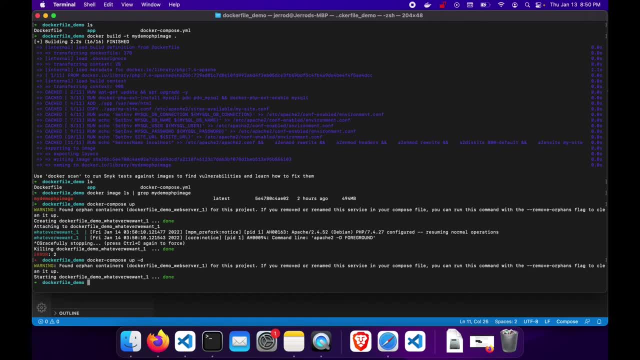 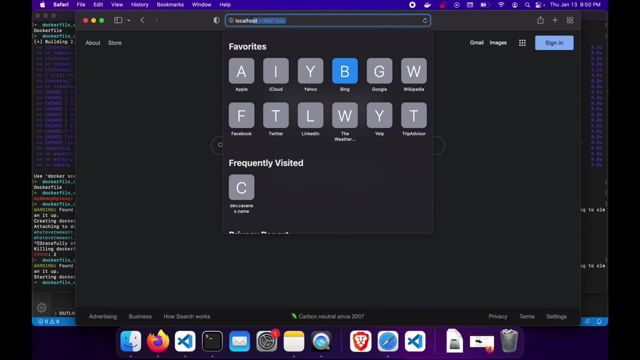 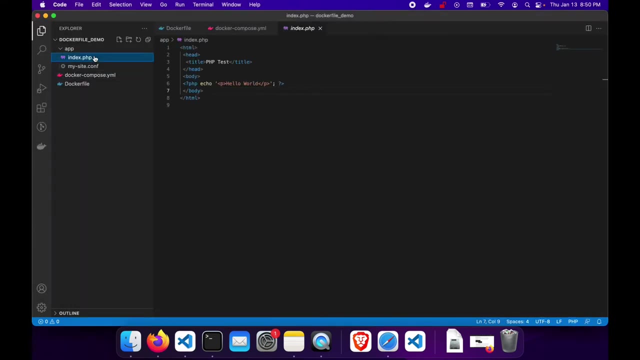 your docker container running in the background. you can choose to you know, go into it if you would like, or just access it from your local browser. so there we go. there's our hello world text. that was the text that was added to our very basic PHP application generally, if you run into any errors, if you have, 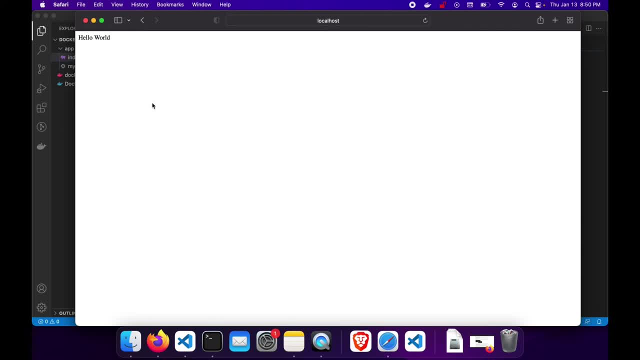 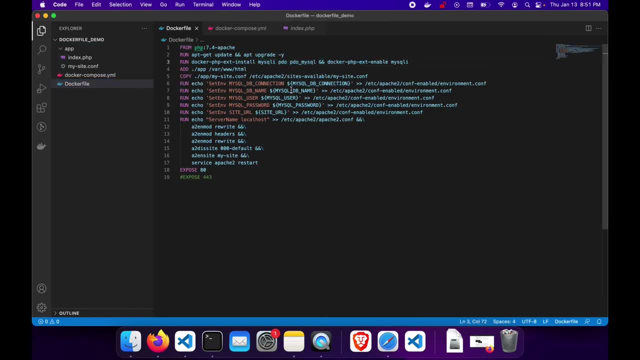 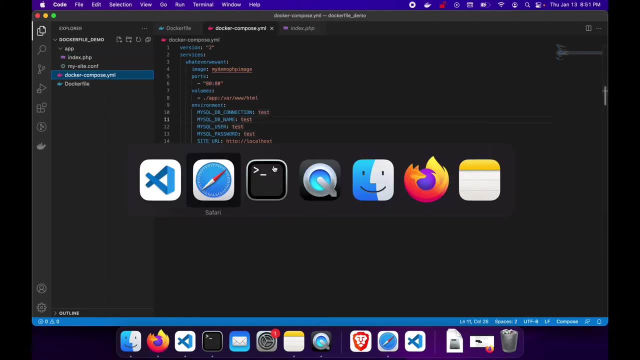 a more complex application, which I'm sure you do. if you're running into any errors saying that you're missing something, you need to more than likely install some additional extensions or update some of your headers or stuff like that that generally comes up when you're dockerizing your container. I just 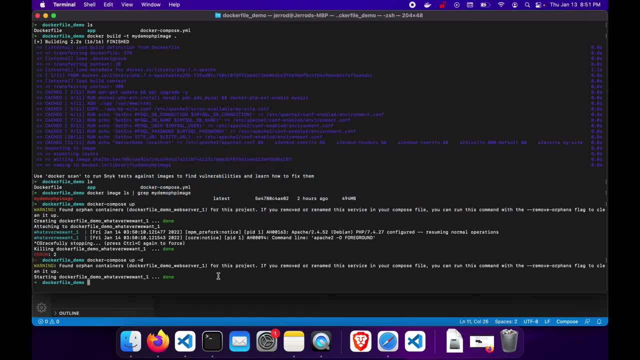 wanted to quickly show that you can actually go in to this docker instance while it's running if you need to do any kind of debugging. so we're just going to run docker ps, which lists the running docker applications, and then I'm just going to reference my image, because I probably have a couple other ones running, right. 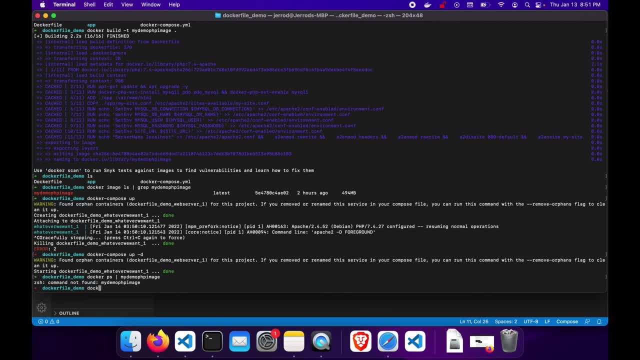 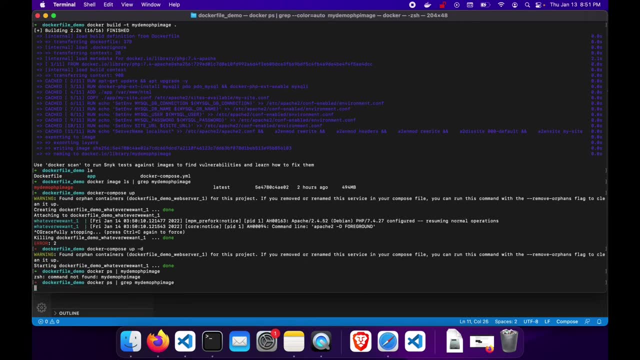 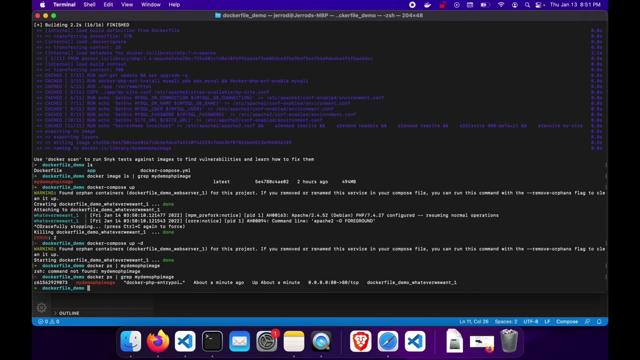 now whoops. okay, so you can go into this docker container that's currently running by running this command. it's docker exec- dash IT and then the name of the docker container which is over here. it's not the name of the image, it's the name of the running container. so we're gonna go. 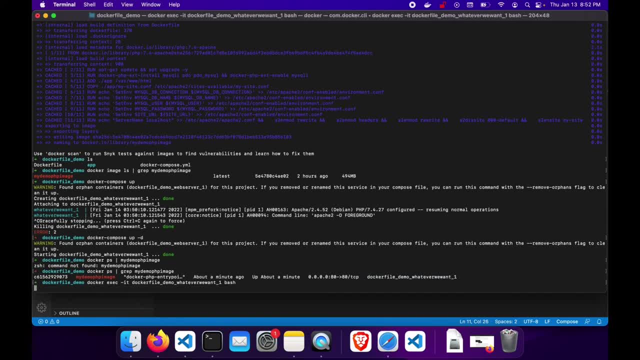 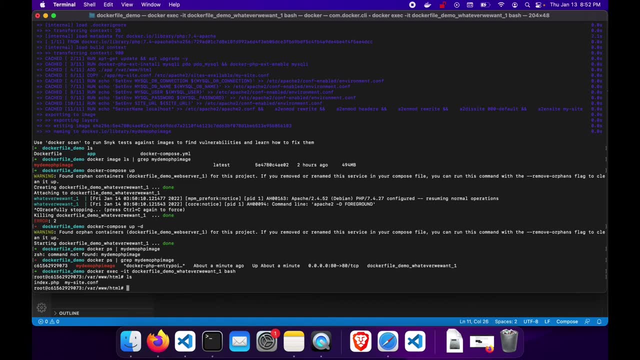 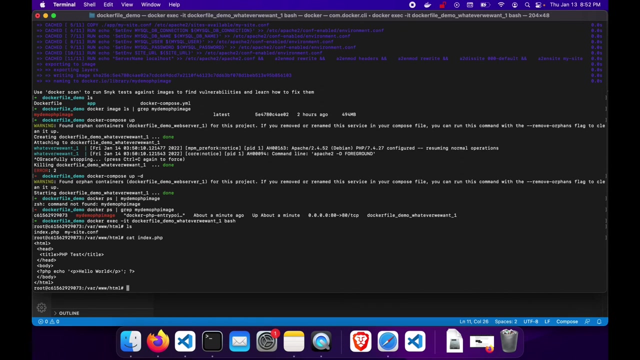 ahead and paste that there, and then a bash shell, and now we're actually in this running Apache docker container, so you can see my site, dot-conf, and then also the index dot PHP file that we had created. keep in mind: if you try to edit any of these files, you're not going to be able. 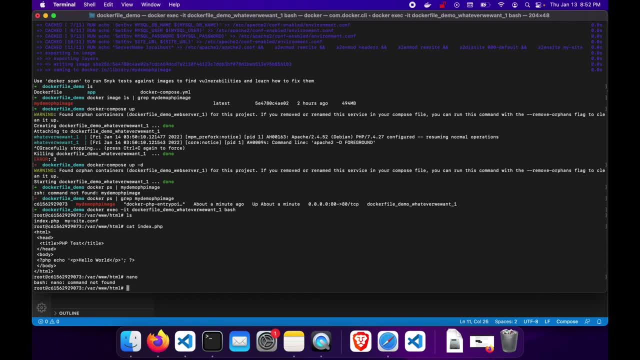 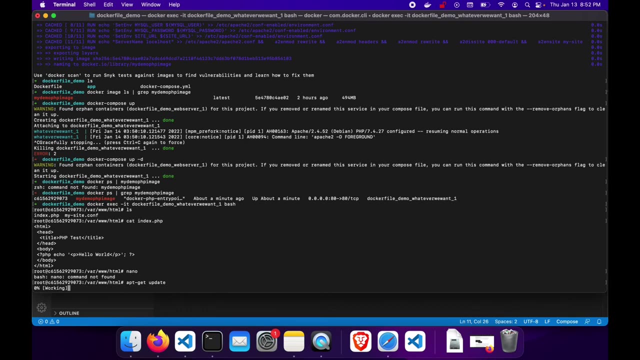 to, as nano is not installed. so what you could do to go buy this. since this is modifying just a container and not the actual image, you can go ahead and install something. if you want to test something out or debug, you can just update the docker container and then just run a AT, ABT, get and 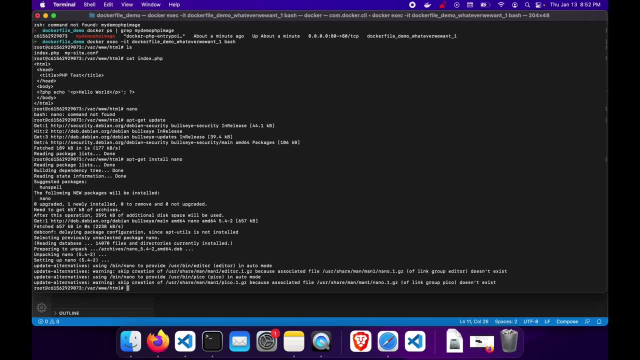 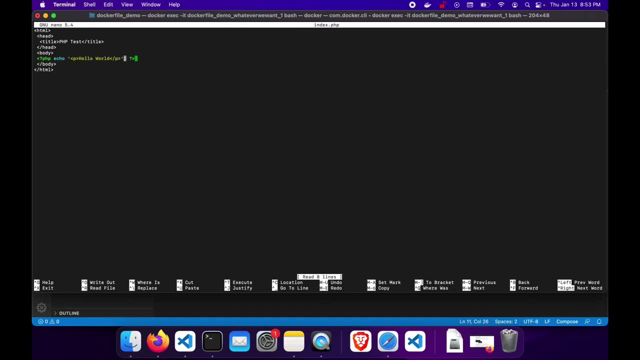 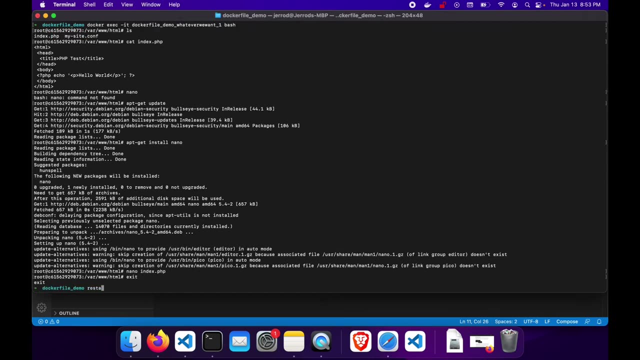 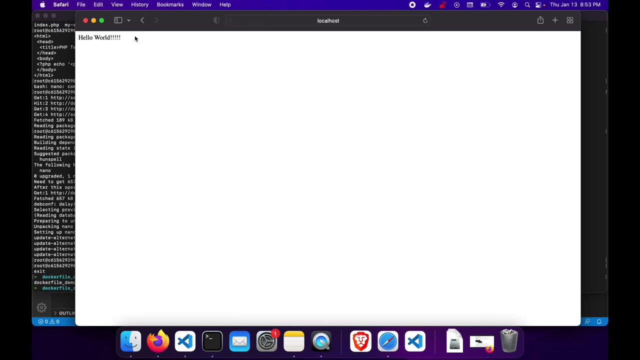 install nano and now you'll be able to edit your file and then, if you want to restart your docker container, you just have to run docker restart and then your container name, and then it'll rerun it and go here, there we go, it's updated, and then you can just stop this container by running. 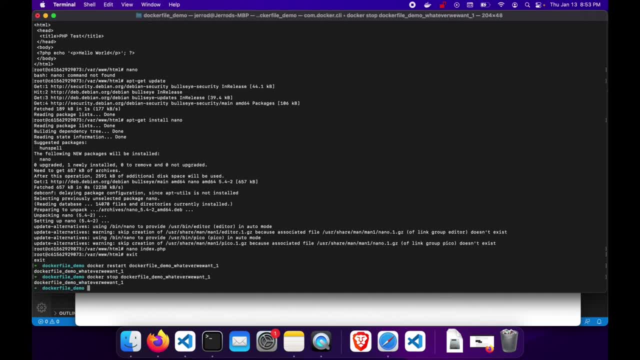 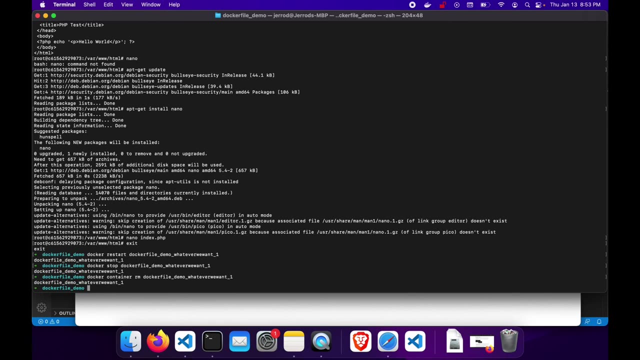 docker stop and then the name of your container, and then, if you want to remove it, it's just docker RM. or you can do docker container RM- it's the same thing, and then it's removed. so now you should know how to dockerize a simple PHP. 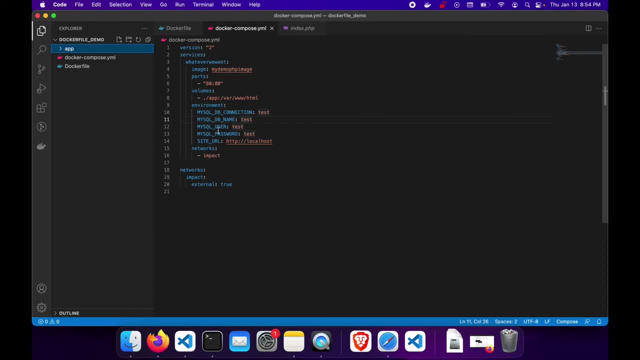 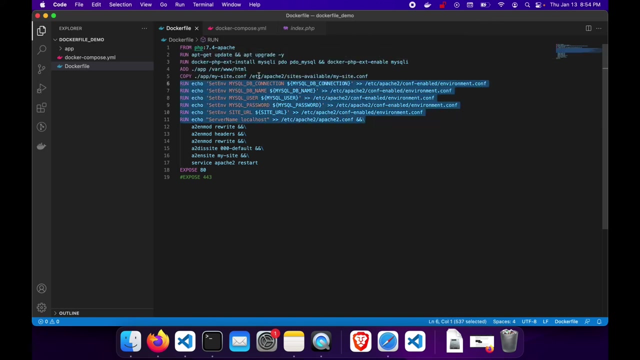 application. basically, if you're doing anything a little bit more complex than this, which I'm sure you're going to be doing, there's just additional things that you can do here. this was just a really bare-bones method that I was using, with some caveats for stuff that I think that you'll be running into, like 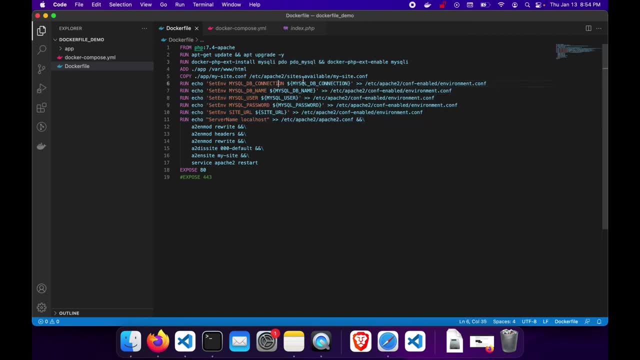 installing extensions, setting environment variables, doing a custom configuration file. you know. exposing to different ports, doing a custom site rather than the default configuration file. you know exposing to different ports, doing a custom site rather than the default Apache service, including your docker compose with your networks for local. 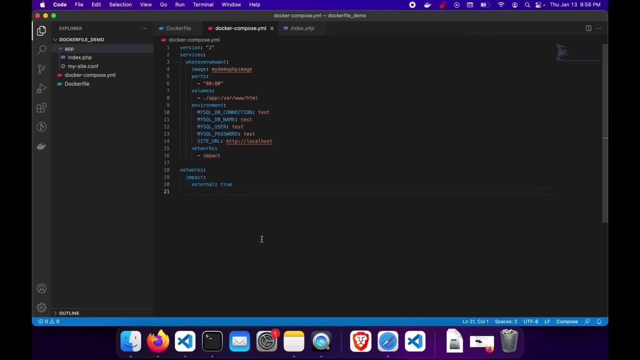 development. just let me know. if you need any help with any of this, leave my contact information in the description. I generally like to do this stuff for clients, so feel free to reach out. thanks,